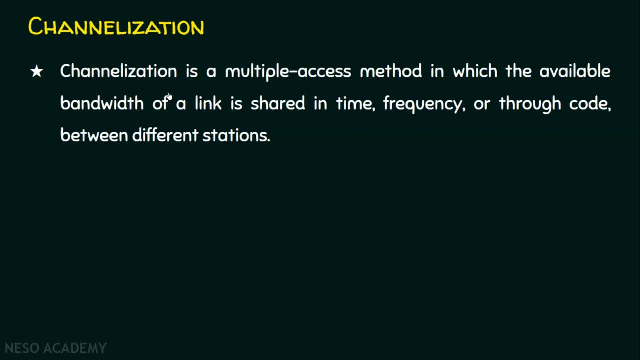 and somehow it was handled in the random access protocols. In the next type, that is, the controlled access protocol method, we use reservation kind of schemes or polling kind of techniques or token passing kind of stuff in order to handle the collision. And the last method is channelization. 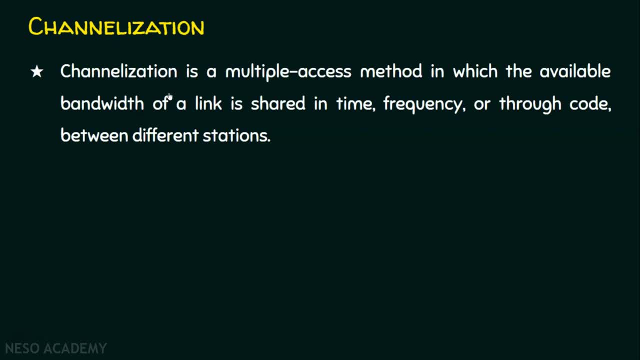 where this entire channel- this entire channel means the entire bandwidth of the channel- is shared in terms of time or frequency or code. Before going into the frequency division- multiple access- let's see what is multiplexing. Multiplexing in computer networking means: 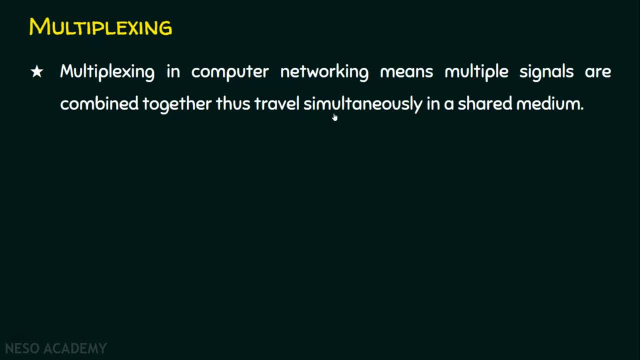 multiple signals are combined together, thus travel simultaneously in a shared medium. So if we have multiple signals, it means multiple stations are sending their signals on a common channel. We are going to combine this together in order to make them travel simultaneously in a shared medium. 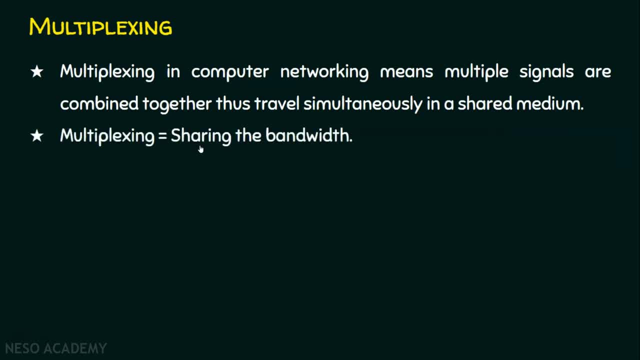 Why do we need multiplexing? Just sharing the bandwidth? When we have a channel, the entire capacity of the channel in terms of bandwidth is going to be divided to multiple stations. Let's see what are the various multiple access techniques. The first multiple access technique: 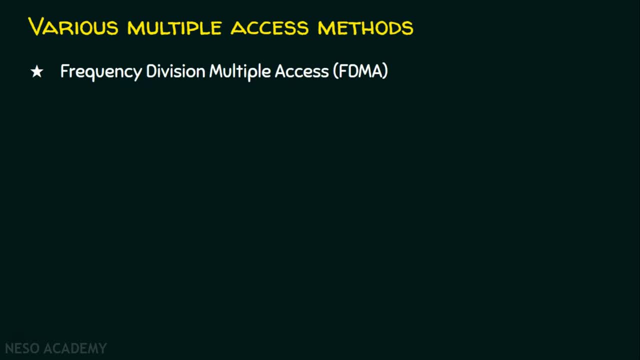 is FDMA, that is, frequency division- multiple access. Second one is the time division- multiple access. And the last one of the session is the code division- multiple access. So we have basically FDMA, TDMA and CDMA. Let's start with frequency division- multiple access. 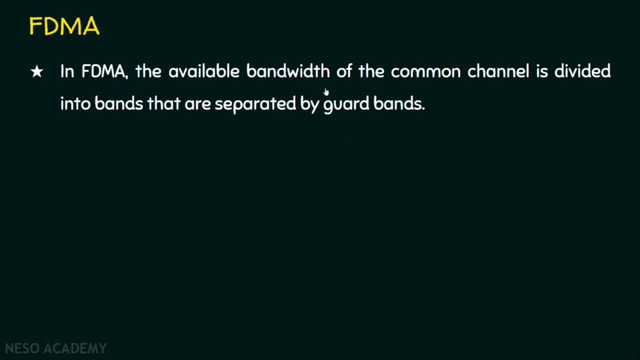 So in frequency division, multiple access, the available bandwidth of the common channel is divided into bands that are separated by God bands, Say, for example. if we have a common channel, we are not going to just click that send the data where this entire bandwidth is going to be divided into bands. 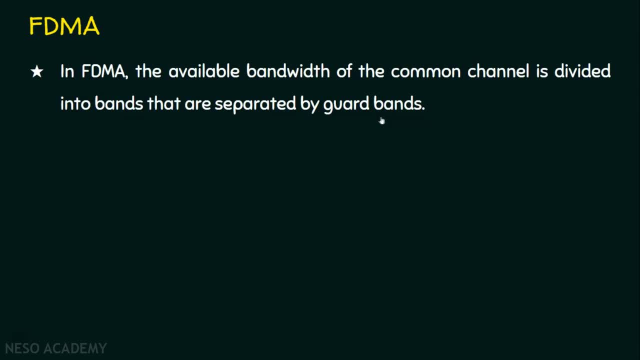 Suppose, if there are five stations, then the entire bandwidth is divided into five user bands and each user band is assigned to each station so that all stations can transmit the data simultaneously. You may ask me a question: what if these two bands are very near? 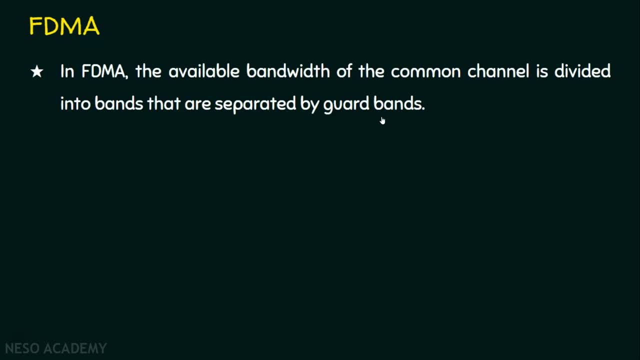 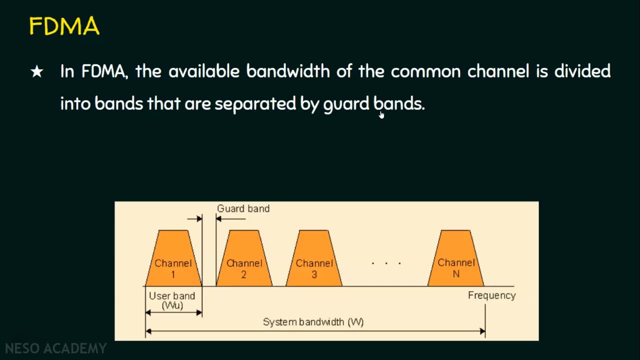 It leads to collision or overlapping. In order to avoid this situation, where each user band is separated by some God bands, we will see the data. So in this diagram now it will be more clear. So in this example, this is what the entire bandwidth. 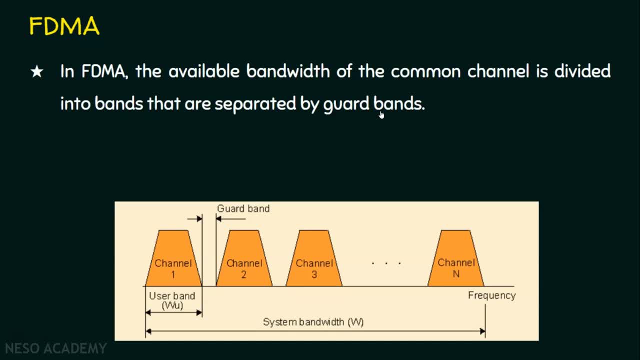 Now this entire bandwidth is shared among n stations, So we are going to create some n internal channels, like channel 1, channel 2, channel 3 up to channel n. Actually, this is only one channel and we are going to break this entire channel into some user bands. 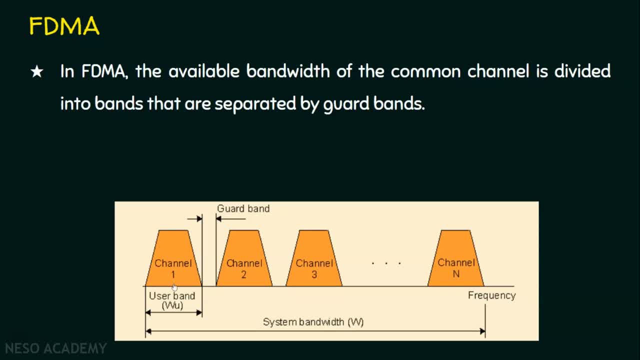 That is what this, this common channel, is divided into some bands, and each band is assigned to each station so that each station can transmit their data at the same time. In order to avoid overlapping of channels, we use a God band, That is, this frequency or this space will not be used. 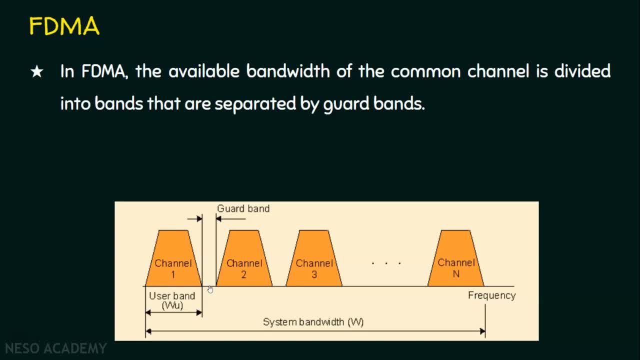 and this is obviously wasted because we don't want overlapping of channels. We will see the next point. So the available bandwidth is shared by all stations. The FDMA is a data link layer protocol. Yes, of course we are talking about media access control. 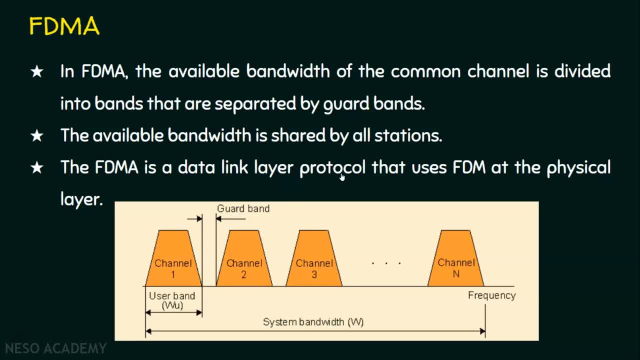 So FDMA is a data link layer protocol, but actually FDM is the technique that is Frequency Division Multiplication. It is not done at data link layer, It is done only at the physical layer. In terms of protocol, FDMA is actually a data link layer protocol. 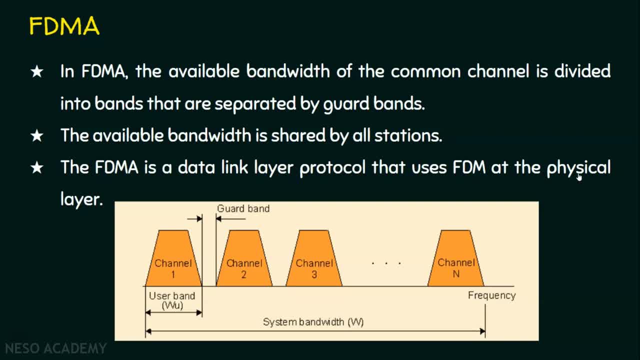 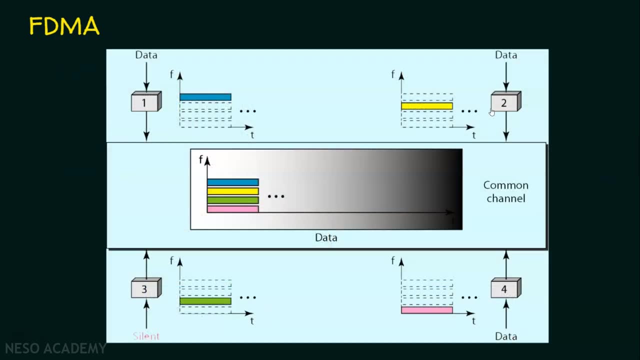 but actually FDM is used at the physical layer because only in the physical layer the data is transmitted as signals. So FDM at physical layer. We will see an example of FDMA now. Suppose if there are four stations: station 1, station 2, station 3 and station 4. 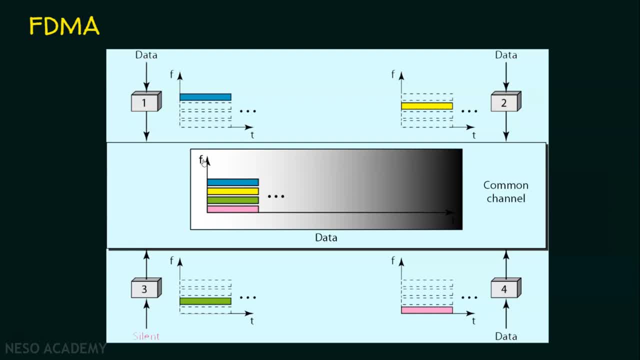 and each station is just one station. How many stations are generating the data? If you observe, this is the common channel. So we know this is the common channel and this end-tab bandwidth is broken into some user band. How many stations are participating here? 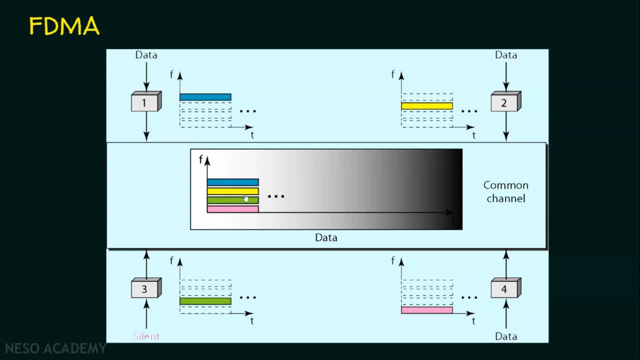 Four, So four bands are created and we also have a guard band here in order to protect it from overlapping. All four stations' data are being transmitted at the same time. If you observe, this blue color data is generated by station 1.. 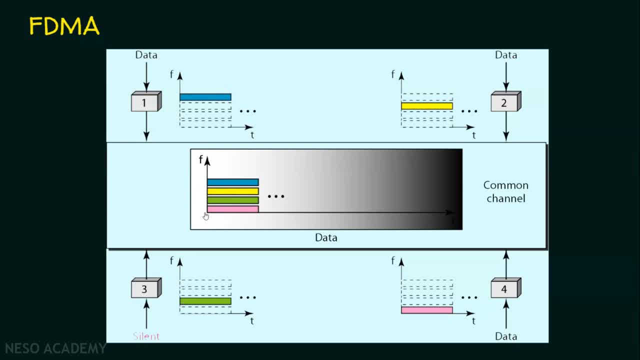 This yellow color is generated by station 2 and this green color data is generated by station 3 and this pink is generated by station 4.. This end-tab bandwidth is used by all stations simultaneously And this user band is for station 1 and the second user band. 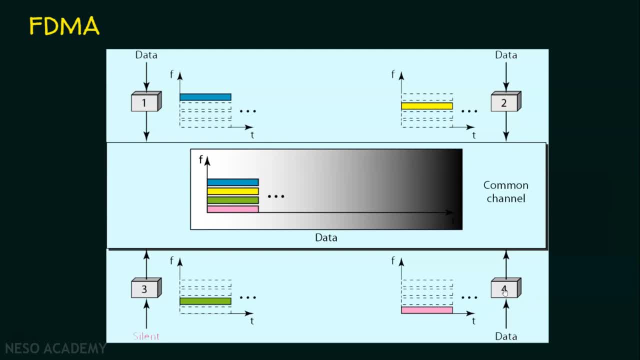 is for station 2.. The third user band is for station 3 and the fourth user band is for station 4.. Thus, multiple stations are transmitting their data at the same time, without collision and without overlapping of data. Now coming to the next technique. 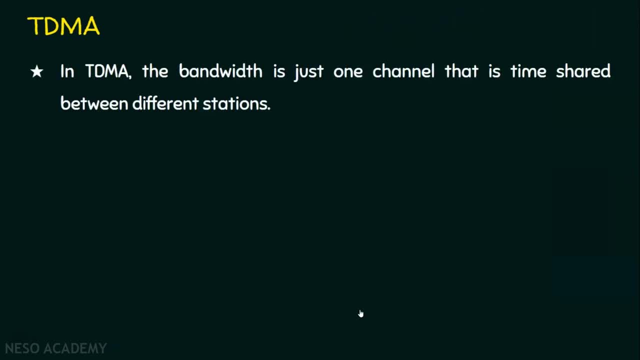 that is the time division, multiple access, where the bandwidth is just one channel. It means the entire bandwidth at that particular time is given to one station only. So the bandwidth is just one channel. that is time shared between different stations. So if we have 10 stations, 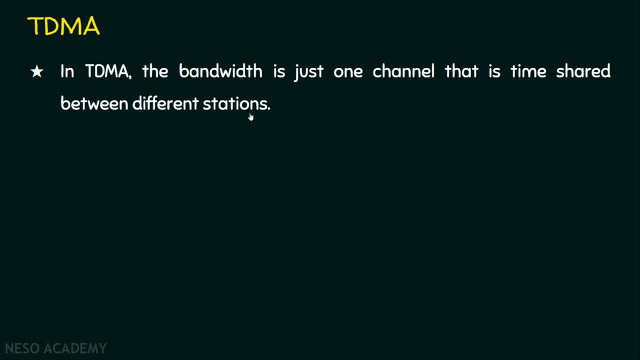 all 10 stations will not send their data at the same time. Rather, each station will be alerted at time, and that time that station will transmit. Let's see it now. So the entire bandwidth is just one channel. It means the full capacity of the channel. 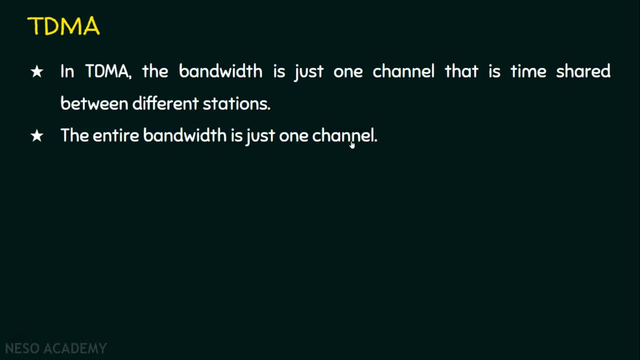 or the bandwidth is given to one station at that time. After that it will be given to other stations so that each station will be using this channel in a time shared manner. So stations share the capacity of the channel in time. We will see the diagram. 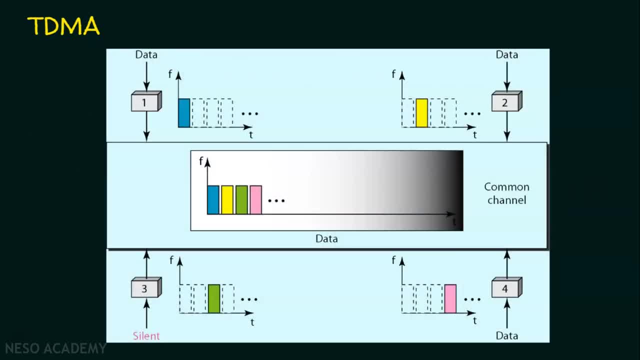 It will be understandable for you. In the previous example we have seen FDMA. Now we will see TDMA. See, if you observe, this time, station 1 is using and the second time, that is, at this time, station 2 is using. 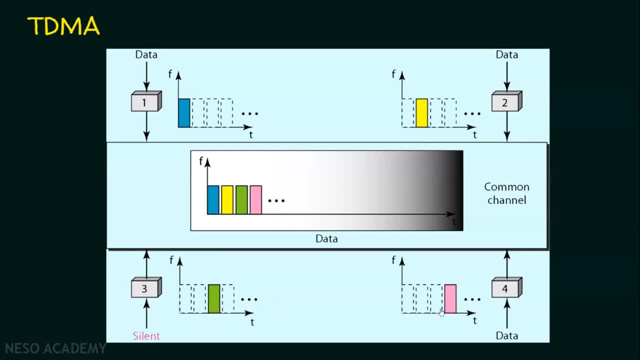 The third time or the third second. for example, station 3 is using, and this time station 4 is using the channel. So, if you observe, not all data are transmitted at the same time in the channel, where the time is allotted to every station. 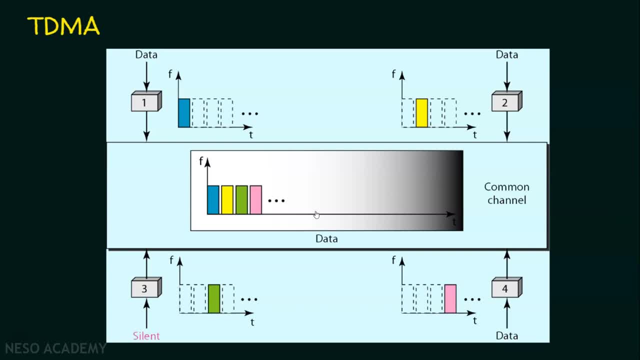 so that that time each channel will use, The entire channel is given to one station and after transmitting that data it will be given to the next station and it will be shared. So TDMA is a time shared approach. Let's compare it with FDMA. 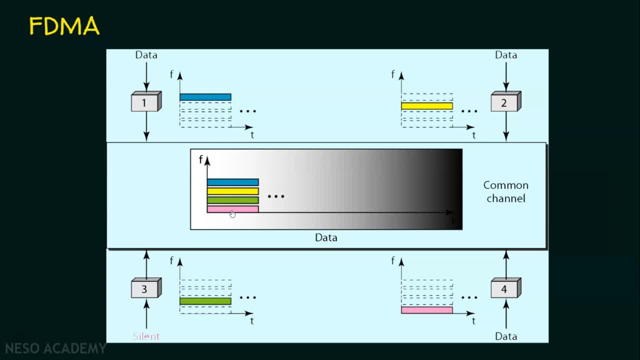 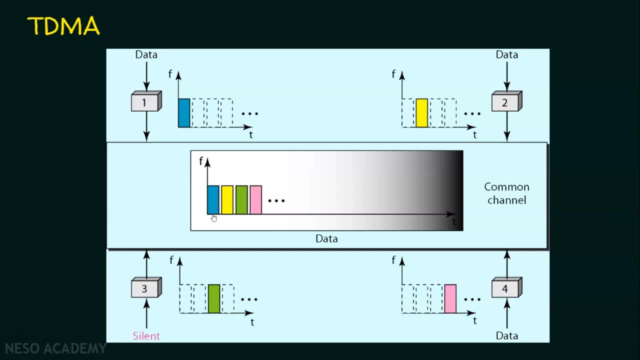 In FDMA, at the same time, all station's data are transmitted, Whereas in TDMA, at a particular time, only one station will be using the entire bandwidth of the channel. Now let's see the last technique, the CDMA. 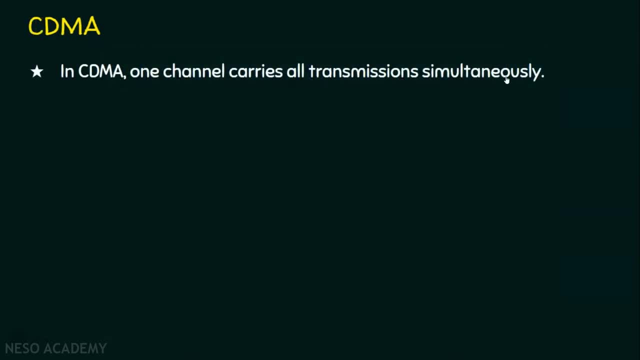 In CDMA one channel carries all transmission simultaneously. It means in FDMA we saw one channel carries all transmission simultaneously. In TDMA it used time sharing approach. How does CDMA differ from FDMA and TDMA? TDMA differs from FDMA because 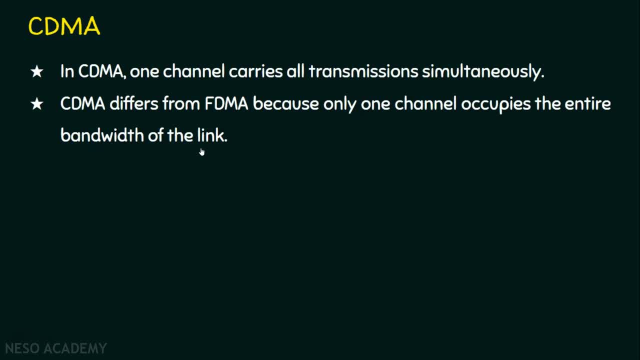 one channel occupies the entire bandwidth of the link Means, at one fine point of time, one channel is occupying the entire bandwidth of the link. Then how does it differ from TDMA? It differs from TDMA because all stations can send data simultaneously. 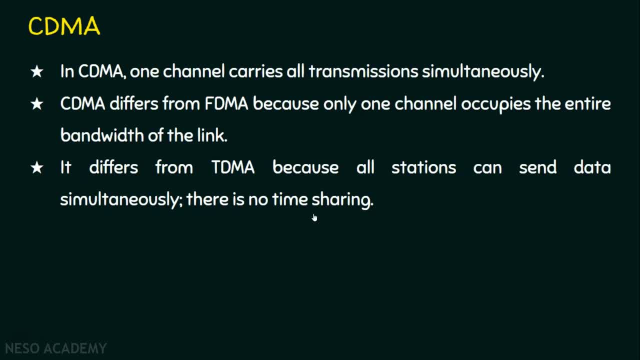 and there is no time sharing. It means at a particular point of time everyone's data will be there in the channel. When we see an example, it will be more clear for you. So in this example there are four stations. station 1,. 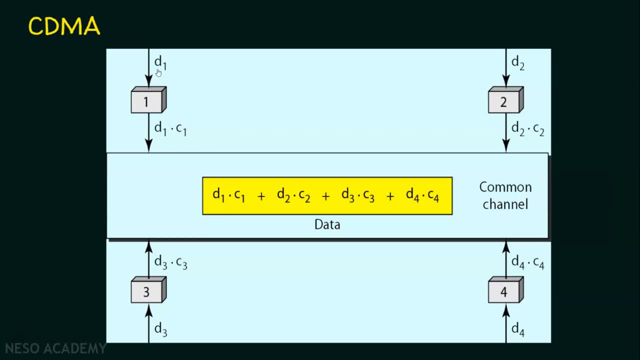 station 2,, station 3 and station 4.. As usual, station 1 is generating D1 data, station 2 is generating D2 data, station 3 is generating D3 and station 4 is generating D4 data. Now each station. 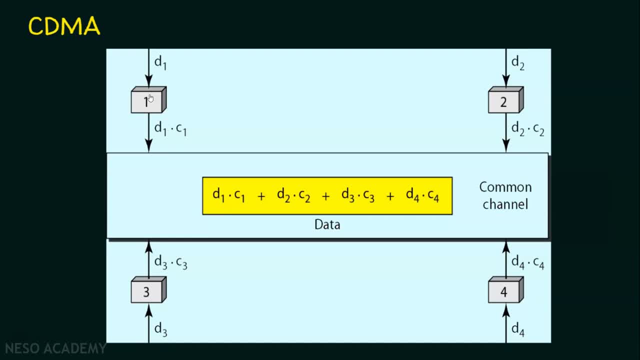 will be having a code. Say C1 is the code for station 1.. What this station 1 actually generates is D1, C1.. That is, C1 is the code. It is applied on the data D1.. Similarly, station 2. 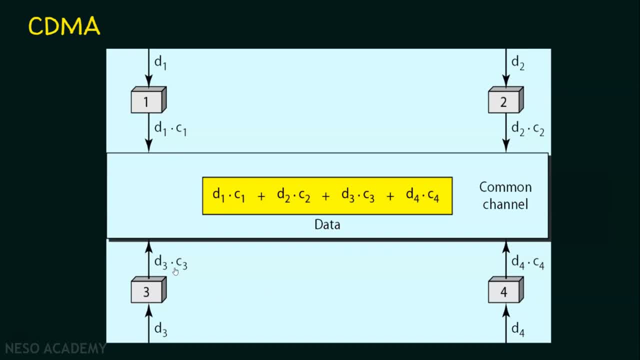 uses C2 code, which is applied on D2.. Station 3 uses C3, which is applied on D3 data, and C4 is the code of station 4, which is applied on data D4. When we see the common channel, all data, that is, D1, C1 plus D2. 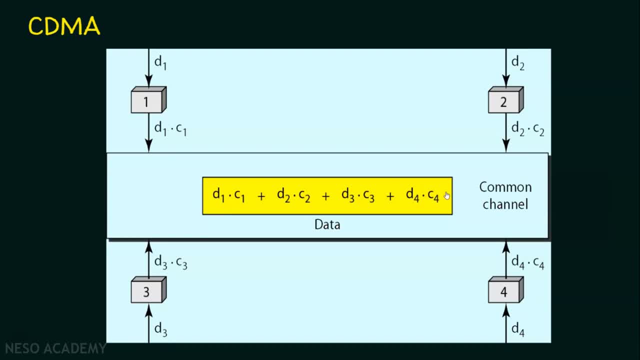 C2 plus D3, C3 plus D4, C4 and all the data are conglomerated and sent as a single data over the channel. So here this is multiplexing, because multiple signals are converted into a single signal. So this is multiplexing. 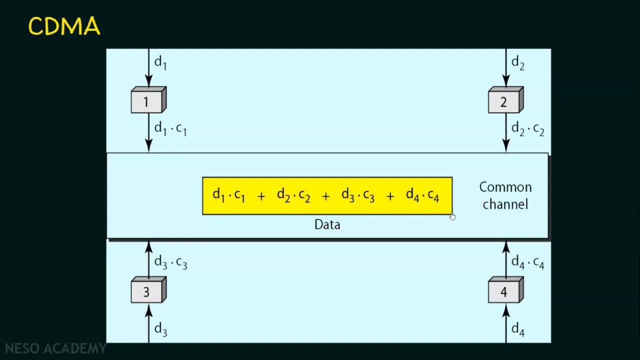 No worries, the receiver will use the code in order to retrieve its data When we talk about this code. actually, these codes are based on the coding theory. I am not going into the details of the coding theory. I am just going to project only two important.